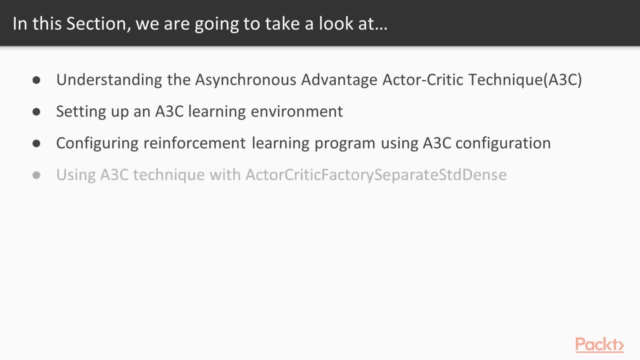 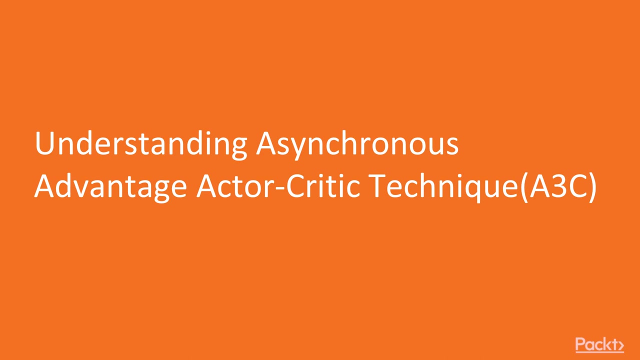 configuration. Here we will do a different approach. Fourth video will be about using A3C training And finally, we'll start our program and we'll gather results. So let's start from the first video, in which we'll be understanding asynchronous advantage, actor-critic technique. So we'll 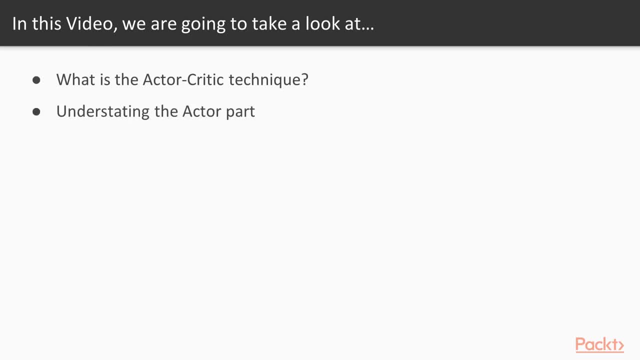 see what is actor-critic technique. We'll be understanding actor part and also be understanding the critic part of our model. So what is that Actor-critic technique? This technique will add yet another concept to our understanding of reinforcement learning. So if you remember from the previous sections, and particularly 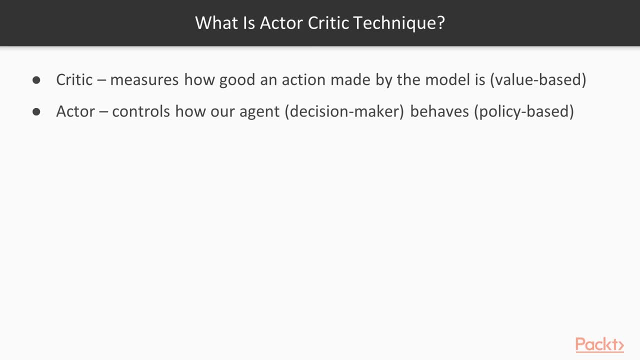 from the section number one when you were explaining the reinforcement learning algorithms. we have state, we have the agent that was an our actor and also we have a reward. There was no, no critic part. Critic part is an another thing that measures how good action. 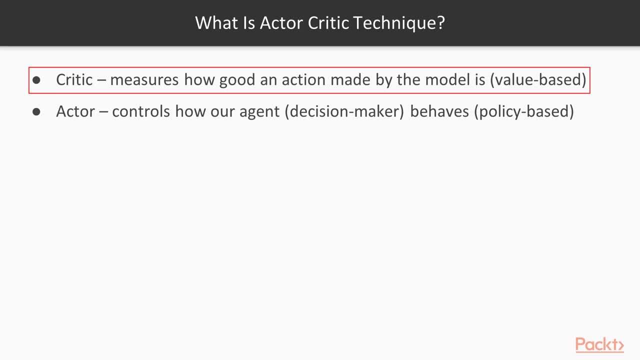 made by model is. So let's see how good action made by model is. So let's see how good action made by model is. So it will take a value into account. Also, we'll have an actor. It will controls how our agent decision maker behaves. 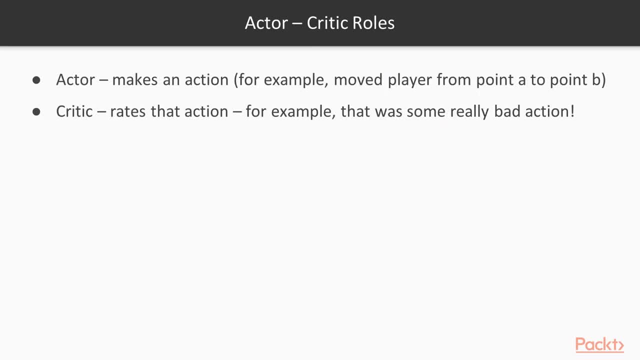 So this will be a policy. Let's take a look at roles of both of them. So actor is made an action. for example, moved the player from point A to point B. So this is responsibility from the actor. It will be influencing the agent. 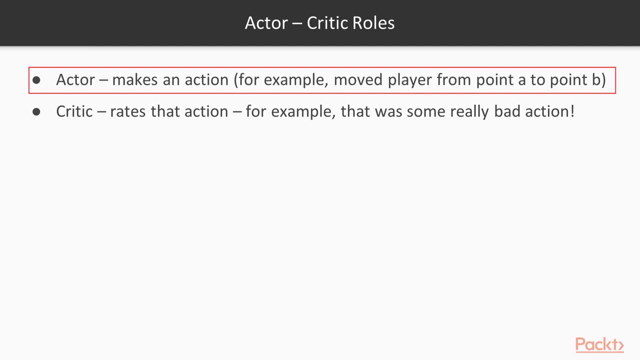 So even remember from the cliff 놓 simulation agent was our player to go from the point A, two, point B, point B. So it will be an actor that will be moving. that agent Critic will rate that action. So when we did an action we'll get a feedback in a way of reward and we will rate it Critic. 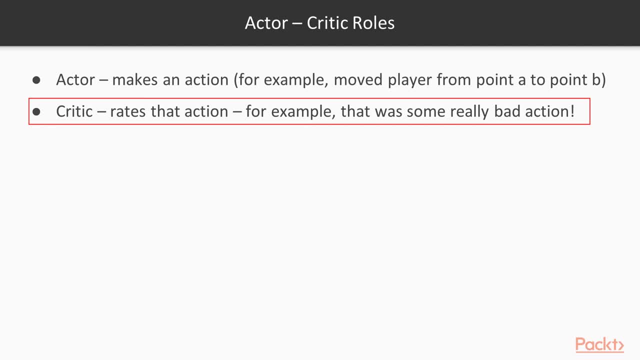 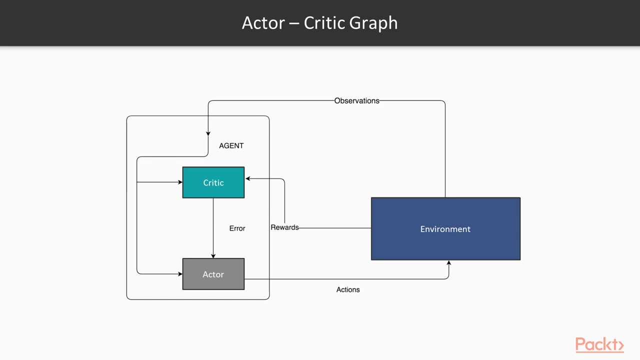 will rate that, and if that is a really bad action, it means that we need to change it. So let's take a look at the graph and try to understand what the actor critics method are. So the critic estimates the value function. This could be the action value or state value. 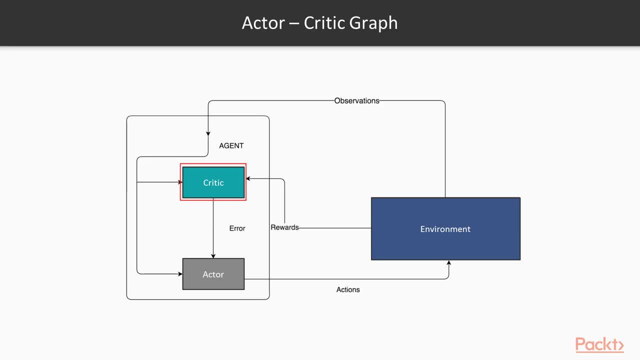 So we can get a state like environment or action. Actor updates the policy distribution in the direction suggested by the critic. So critic is responsible for telling our actor if that was an error or not. So, based on a reward, critic is doing a decision. So